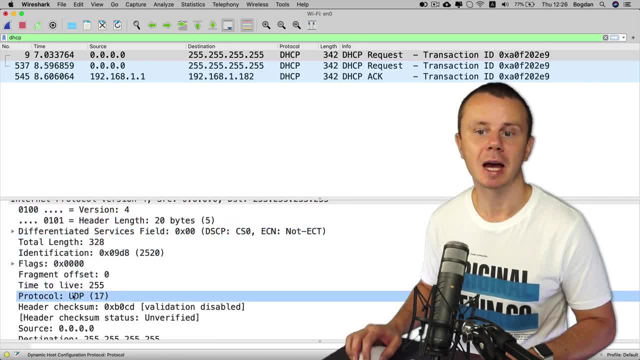 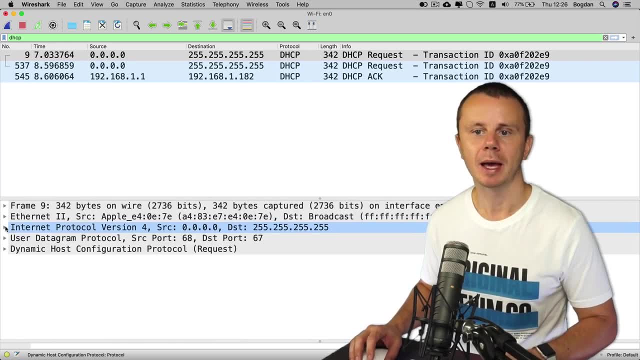 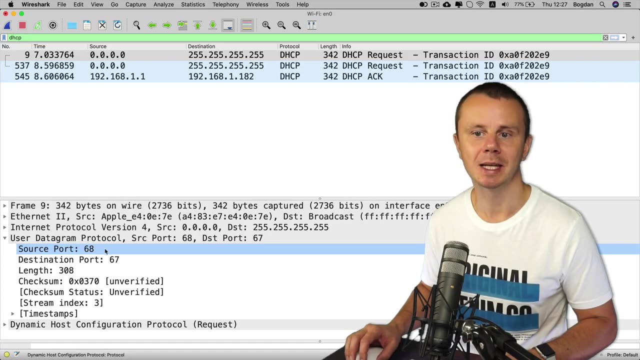 IP version 4 header and inside of this IP version 4 header there is a link to inner protocol and it is UDP in this case. Let's have a look at UDP header, user datagram protocol, and there are just four fields: source port- that is 68. destination port is 67. length is the entire length of UDP. 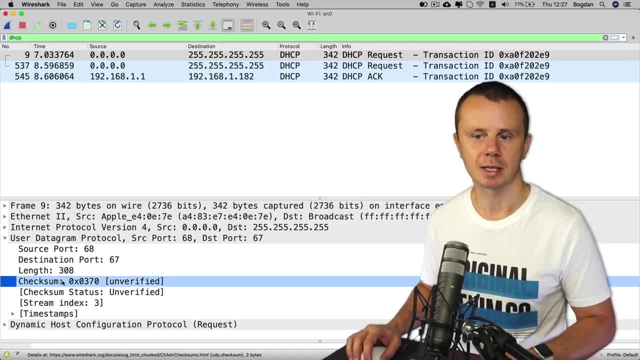 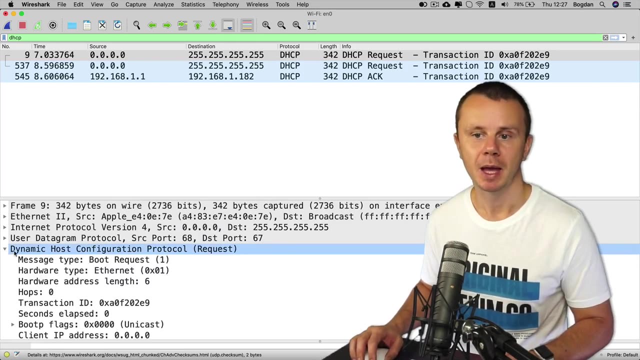 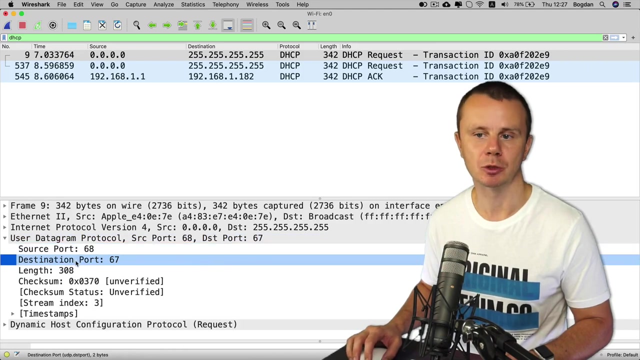 header plus data and here is checksum and that's basically all fields that are included in header of UDP protocol and inside of it there is some application data and in this particular case application layer protocol is DHCP and here inside you may find DHCP request. again. please notice source port and destination port. source port is 68 and destination port is 67.. 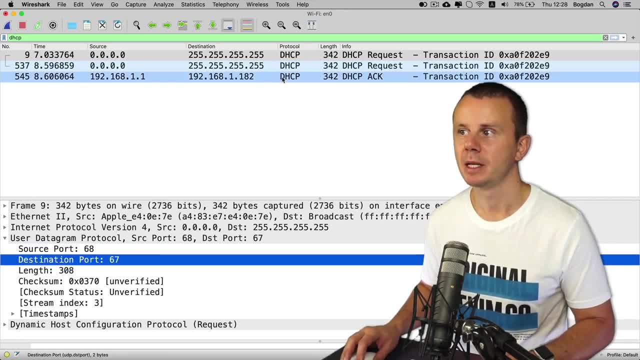 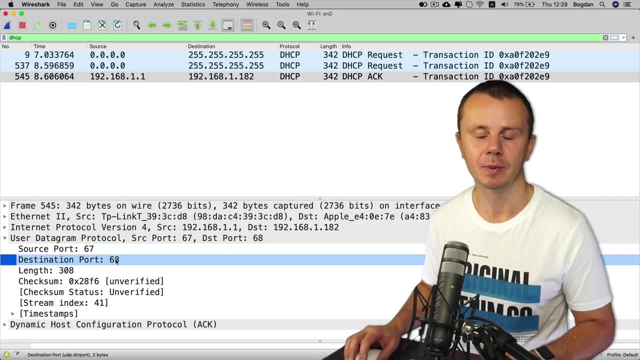 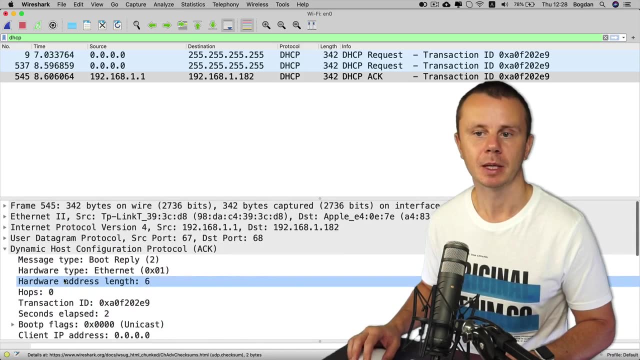 Let's now observe response from the server. here is basically this response that is sent from source port 67 to destination port 68. here is again length and checksum and inside of it there is DHCP related data, DHCP acknowledgement in this particular example. That's how UDP. is used by DHCP. why UDP is used here? because there is no need to establish TCP connection between client and server just for one request for IP addressThat's why UDP is better choice in this particular example. Also, UDP is used for DNS requests. let's here, instead of DHCP type, DNS. 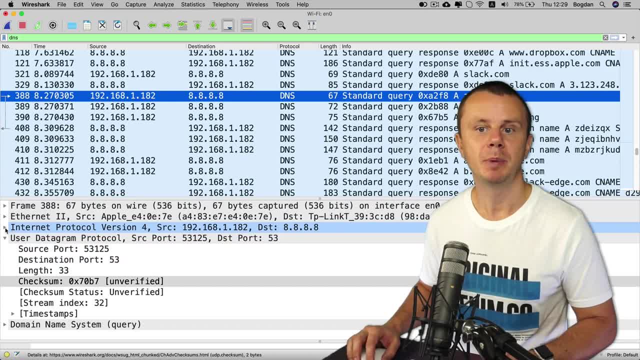 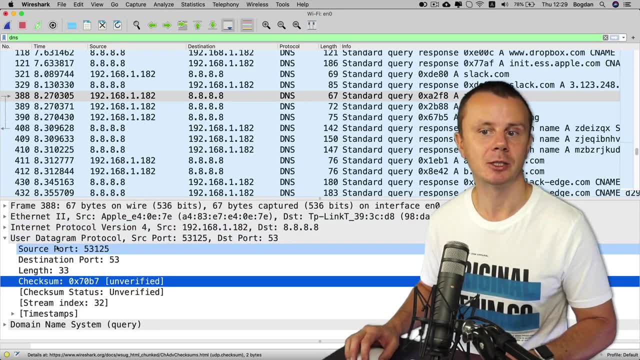 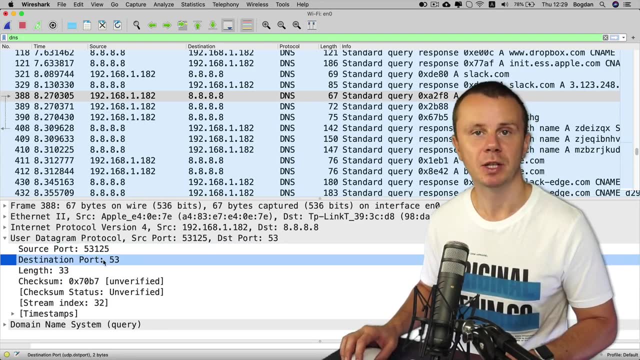 Here again I see UDP protocol In AP version 4 header. I see link to UDP in protocol field And next I see UDP protocol. that again has just 4 fields. source port is random port that was chosen in my case, like this, destination port is 53, it is DNS port length and checksum. 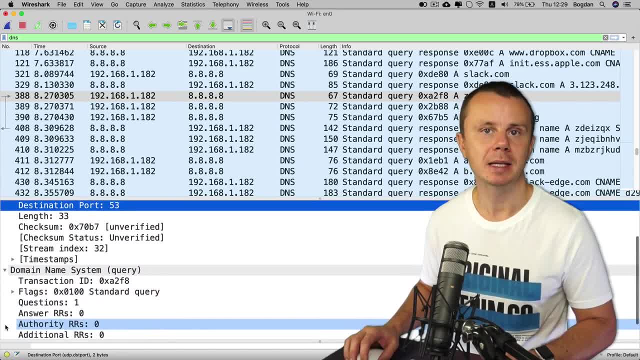 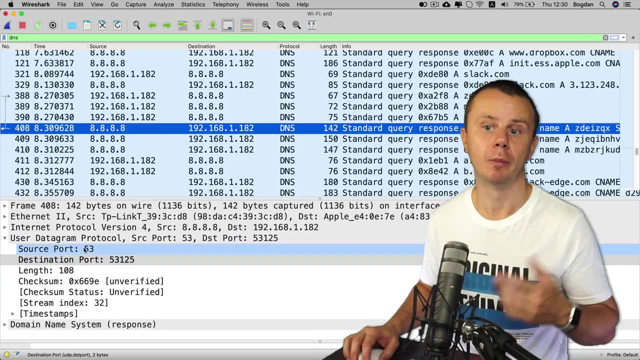 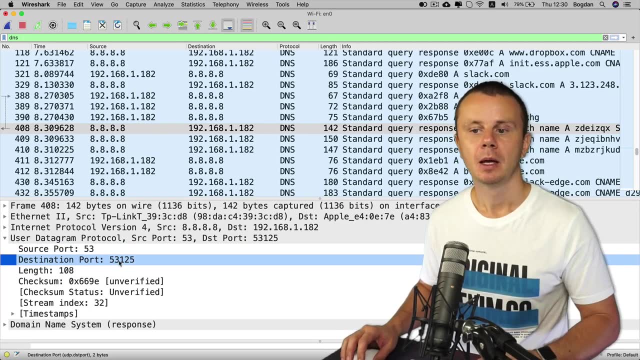 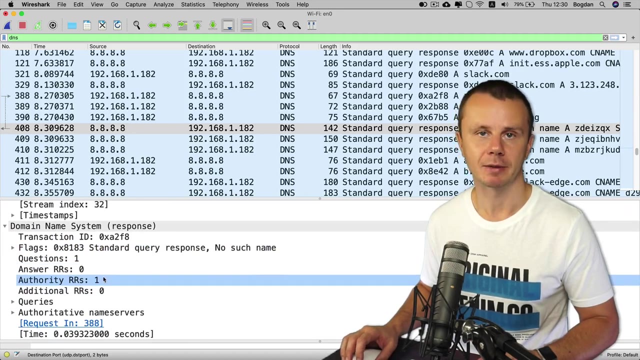 And inside there is DNS related data and DNS is application layer protocol And response from remote DNS server. goes from port 53 to my local port that I used in DNS request And again there is some application data inside. it is actual DNS response from DNS server. 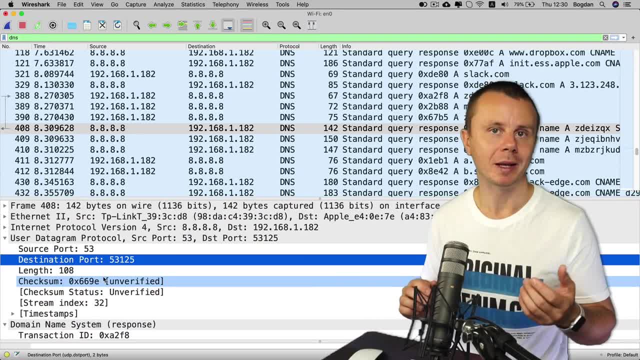 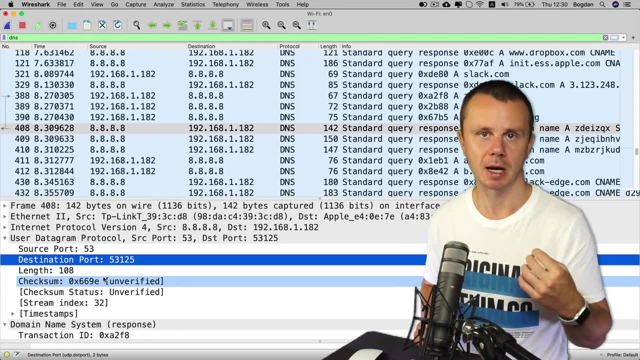 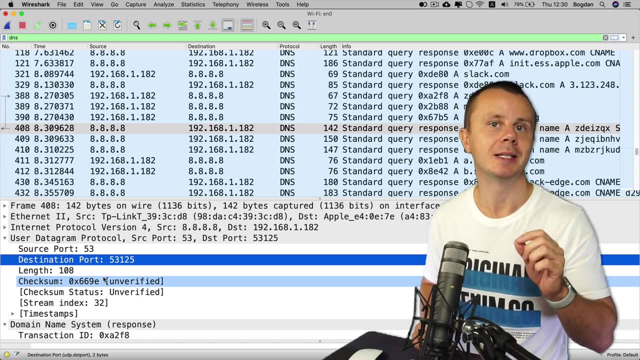 That's how UDP is used for DNS Again. reason why it is used here is that for DNS we usually send one DNS request and receive DNS reply from the server. No need to establish TCP session, no need to tear down it, Because if we were using here TCP instead of UDP, then we would have at least 6 different. 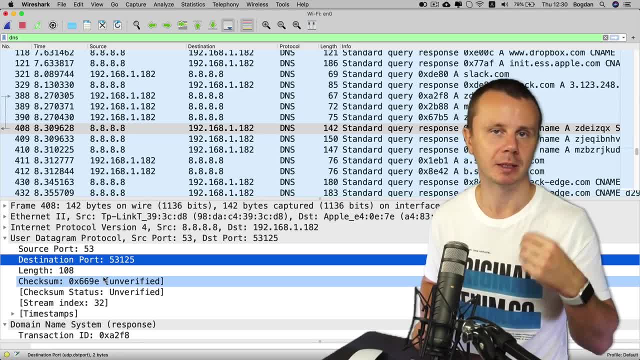 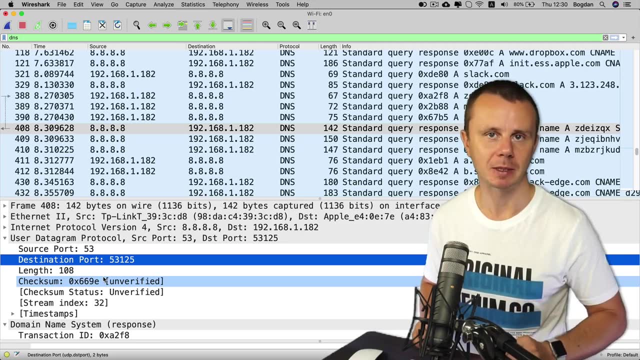 TCP segments: 3 segments for establishment of the connection and 3 segments for tear down of the TCP connection, And at least one segment would be needed for actual data that should be sent from the server back to client. So in total 7 different TCP segments. 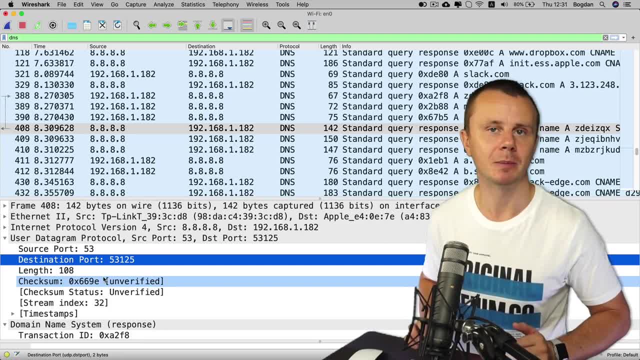 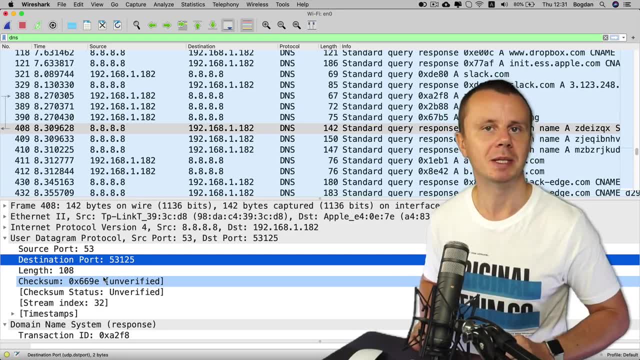 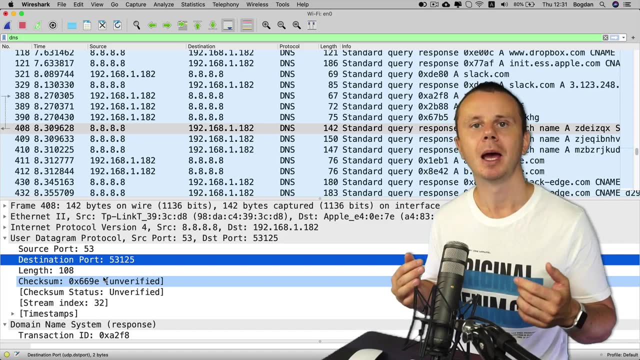 That is a waste of time Because it takes more time than just send UDP request and receive response. Just 2 different UDP segments. That's why for some protocols it is better to use UDP instead of TCP. It is faster and it doesn't require any establishment of the connection. 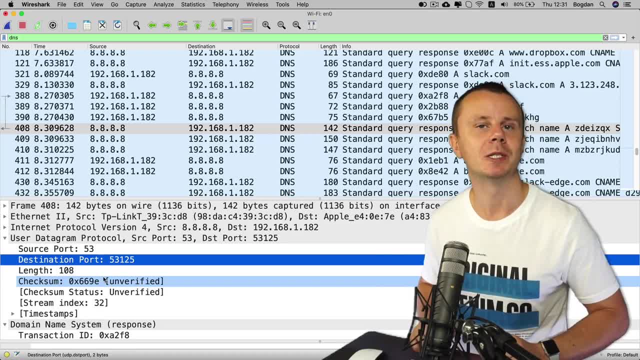 That's all for UDP, and next let's summarize what we discussed in this section.